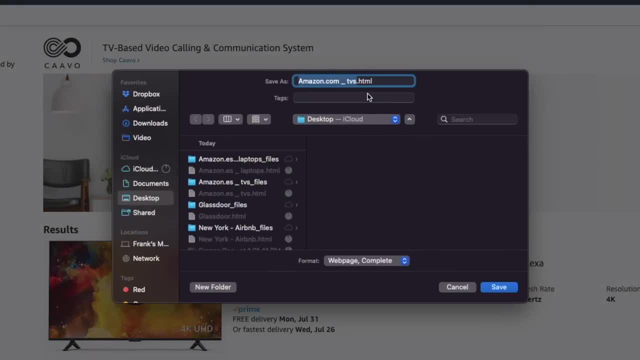 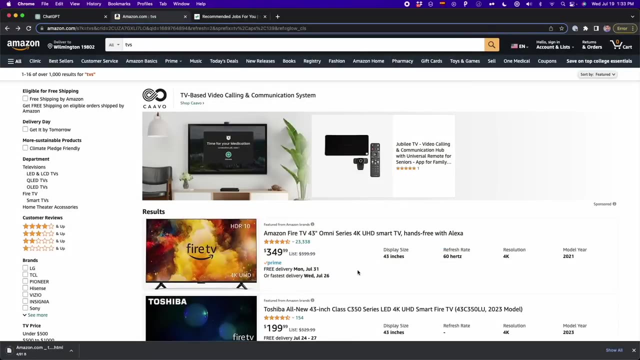 So we're going to save this file as an HTML. So this one is going to be amazoncom TVs and I'm going to save it. So I'm going to press on Save And now I have this file on my computer. then we're going to upload this file to. 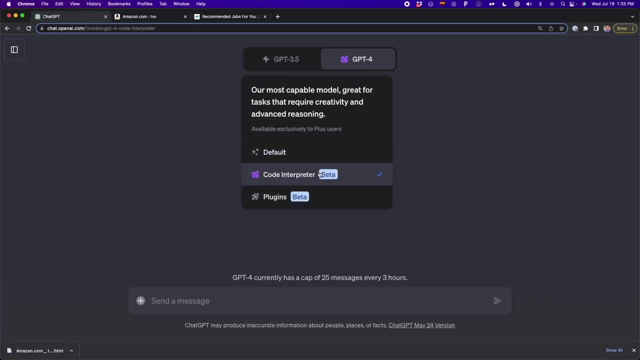 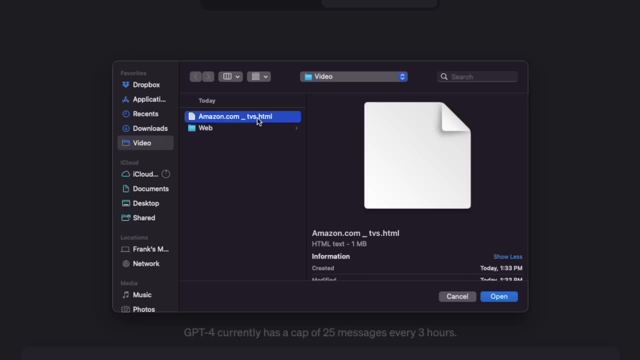 chat: GPT code interpreter. So we go to GPT For we select code interpreter and then we upload this file. So I press this button and then I select this HTML file that we just saved. So here, if I see the preview, we're going to see that website. but now in this, 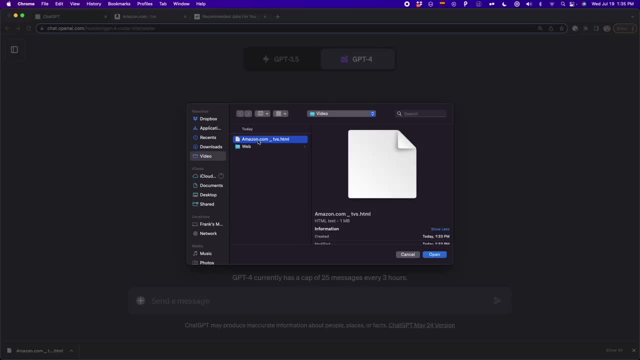 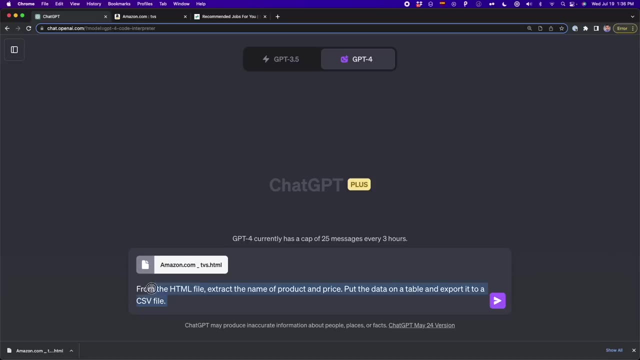 simple HTML format and we have to upload this file to tell chat GPT to extract some elements from this file. And we're going to use the following prompt from the HTML file: extract the name of the product and price And put the data on a table and export it to a CSV file. So, basically, we're going to 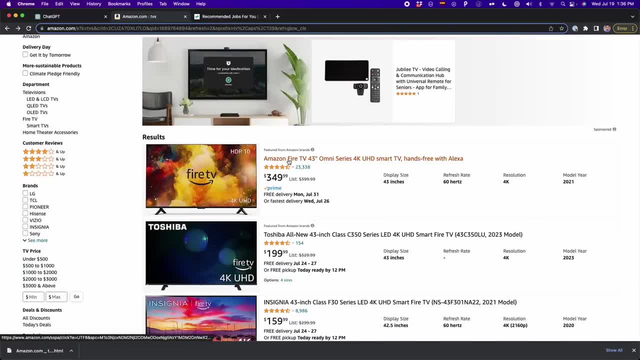 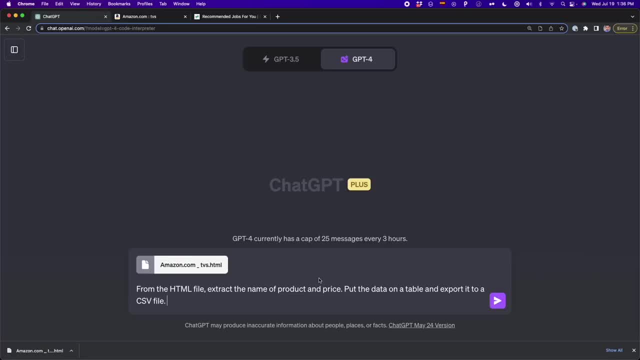 strike only that name of the product, for example, Amazon Fire TV, and then the price: 349.. And then we want to put this on a table and export it into a CSV file. So with this sometimes it's enough, But in this case I'm going to add more details And I'm going to 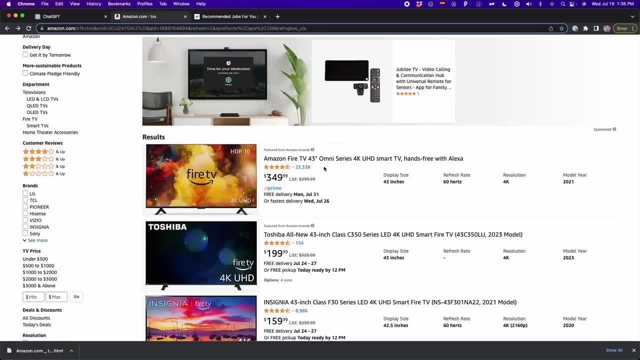 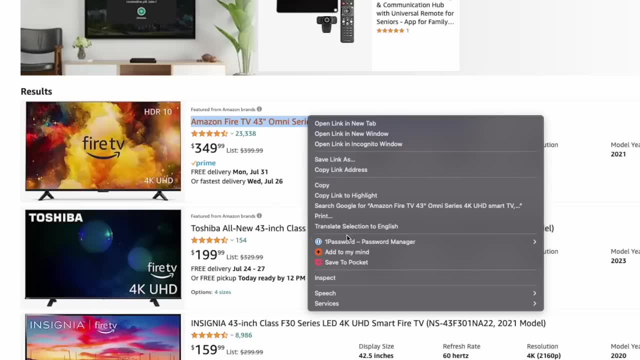 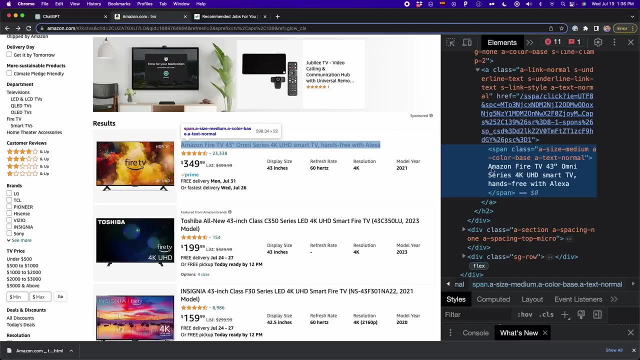 tell. or I'm going to help chat GPT by giving the element where this name of the product and the price is In the HTML file. So here I'm gonna right click and press on inspect And we're going to get this developer tools. So here what we're going to provide is the name of the 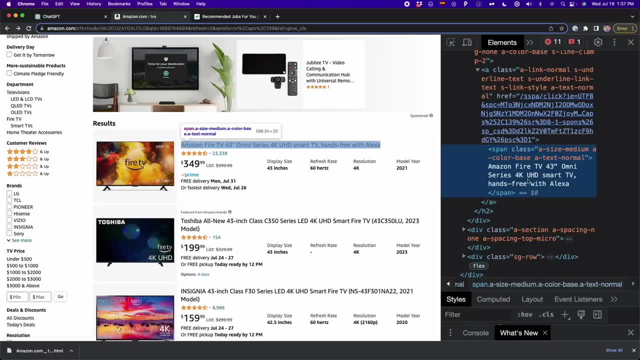 element where this name of the product is located. So in this case is this element, As you can see, if I select this, this name or this element, this is highlighted in blue. So this is the element. So I'm going to copy and I'm going to paste it here. So I'm going. 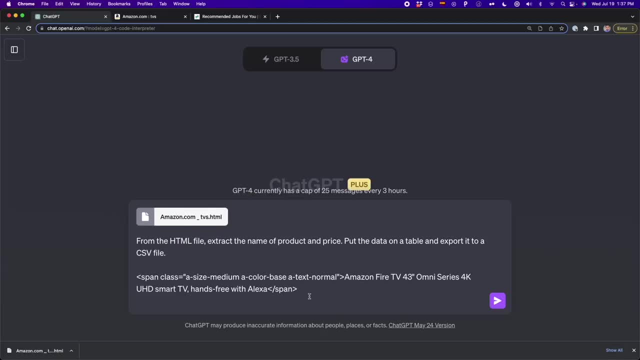 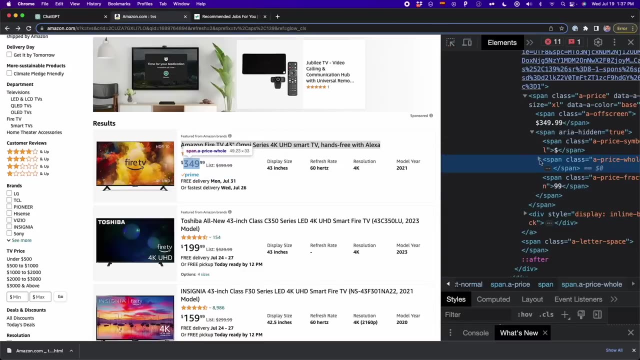 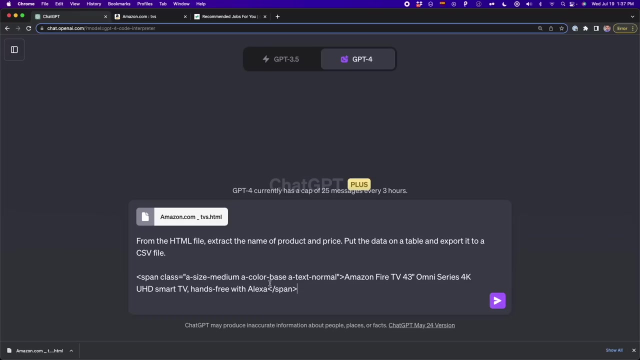 to press here of the product. now we have to continue with that price. so here i select the price and now we have the price which is this one. so i'm going to press ctrl c and then i'm going to paste it below. i'm going to tell now chat gpt that here is the element of one of the products, so it's going to. 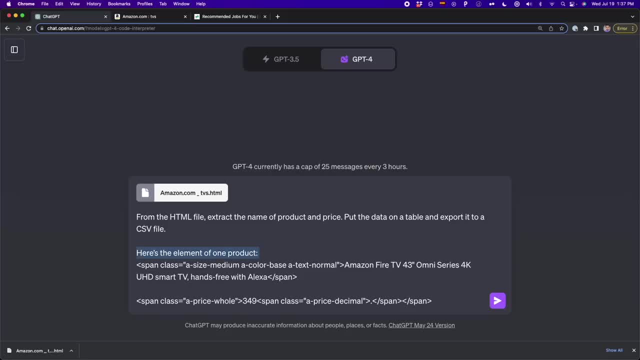 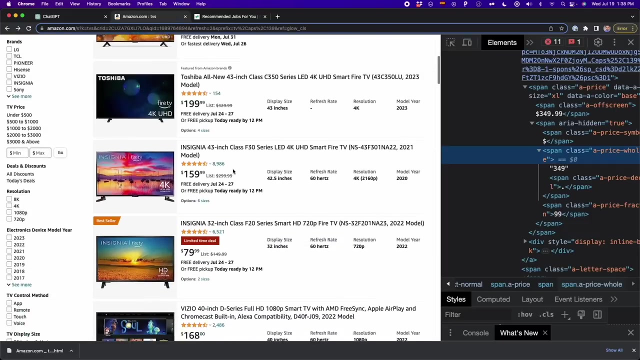 help get the right element. so here i type: here is the element of one product and then i'm going to tell chat gpt that this one is the element of the price. and finally, to finish with this prompt, which is pretty long, i'm gonna deal with the missing data because, as you can see here there are some. 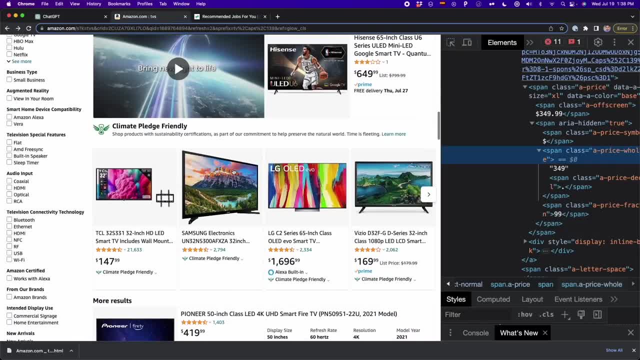 tvs that don't have the price. and in case we don't tell chat gpt what to do, it's going to duplicate the price of other products. for example, here we have samsung electronics and this one doesn't have a price, so probably it's going to duplicate the 157 from this product or the 16. 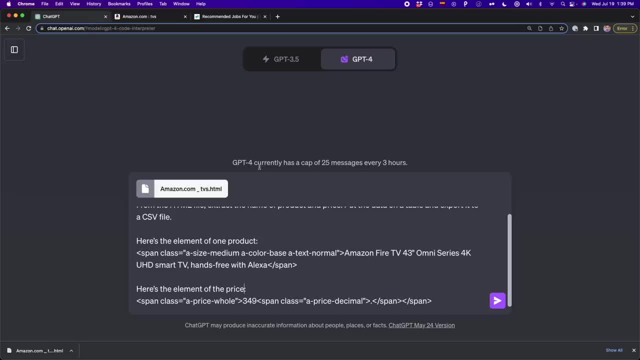 and the 1696 from this other tv. so i'm gonna tell chat gpt how to deal with this missing data. so here i'm gonna tell this: in case the price of the product is missing, just leave that price as a null data and with this we're done. so i'm gonna send this message and we're gonna. 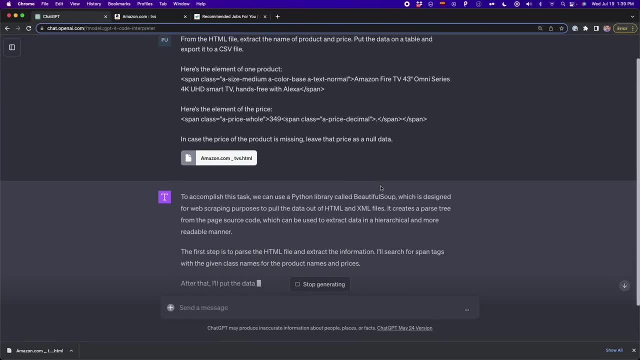 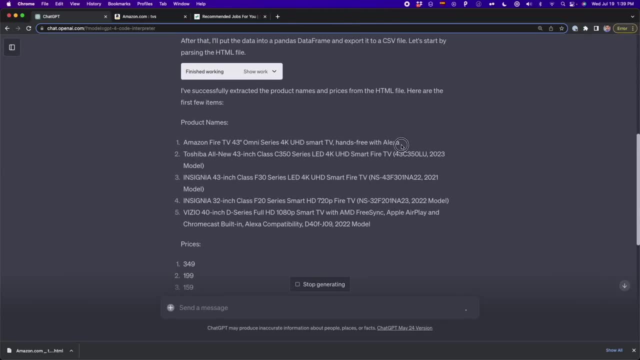 see how chat gpt and the code interpreter is going to do all of this. so, as you can see, chat gpt is extracting the name of the products. for example, here, first we have the amazon fire, and then we have the amazon fire, and then we have the amazon fire and then we have the amazon fire. 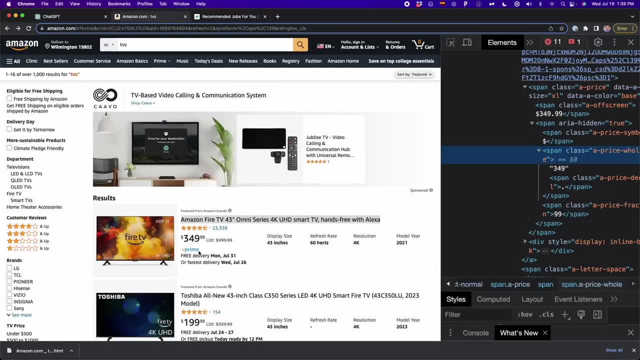 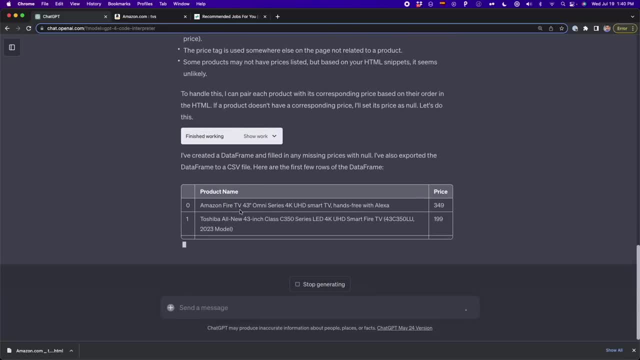 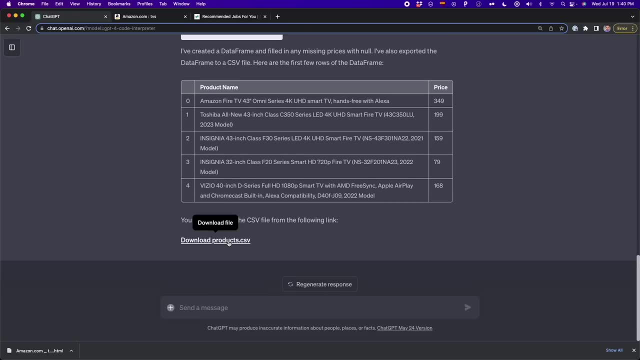 43 inches, and probably this is the first one, yeah, and it's 349 and, as we can see, is the correct price in the correct product. now it's doing some more stuff and, yeah, now it's creating the table that we wanted and we have two columns, the name of the product and the price, and then it's providing. 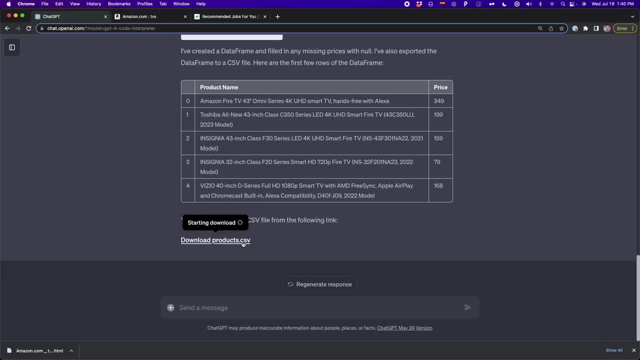 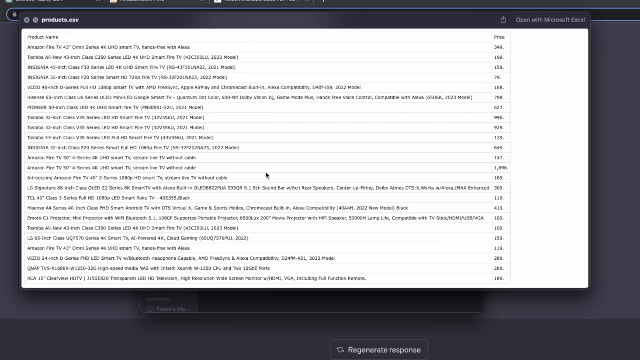 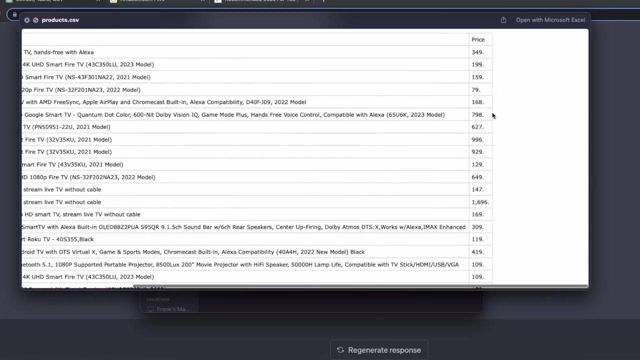 this csv file with all the data script. i'm gonna download this csv file and i'm gonna open it up. so here i have the productscsvchatgpt generated and now we can see all the data script. so we can see the amazon fire tv 43 inches to shiva insignia and more brands, and here we can see the price. 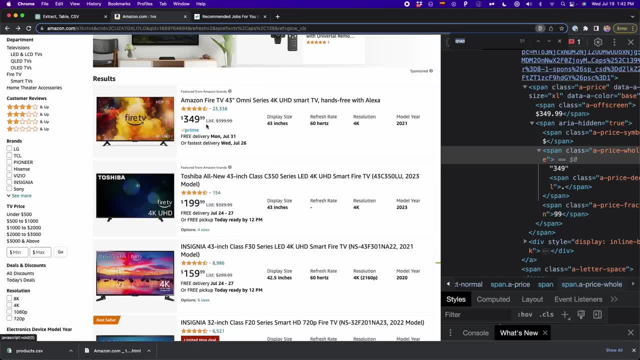 and if we go here, we're gonna see that all the data was correctly extracted and if that's not the case, you can just do some prompting and tell chat gpt what was the mistake, so you get the right data and the data is not corrupted or it doesn't have any issue. and now what i'm going to do is: 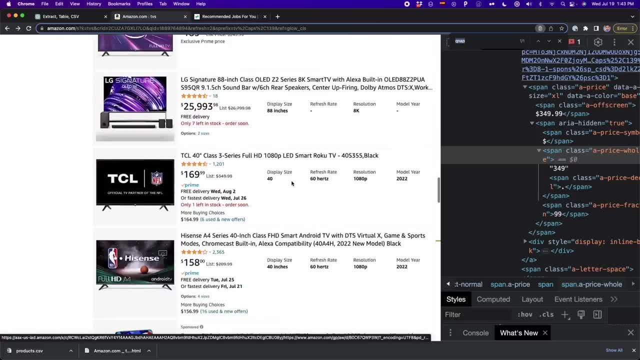 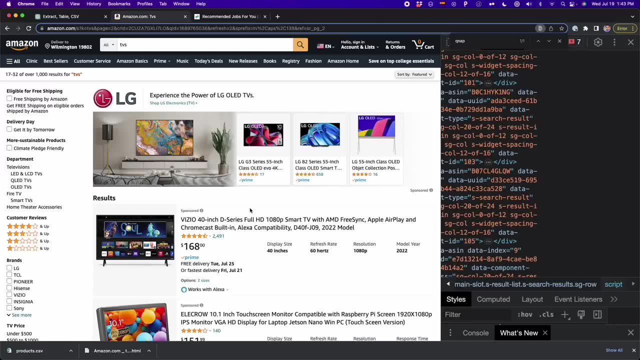 extract the same data, but from that second page. so i'm going all the way down and i'm gonna click on the second page to show you how you can do this in all the pages. i'm going to do an example with the second page. so here i'm going to close this one and i'm going to repeat the same process. 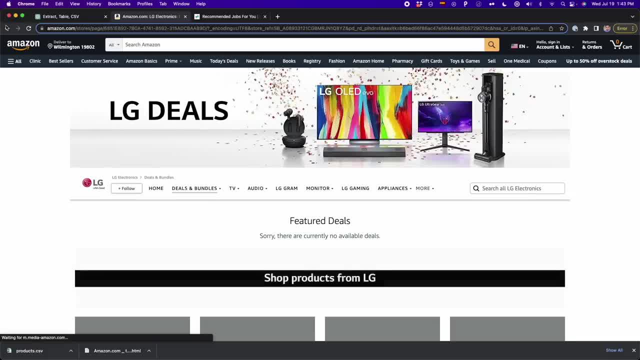 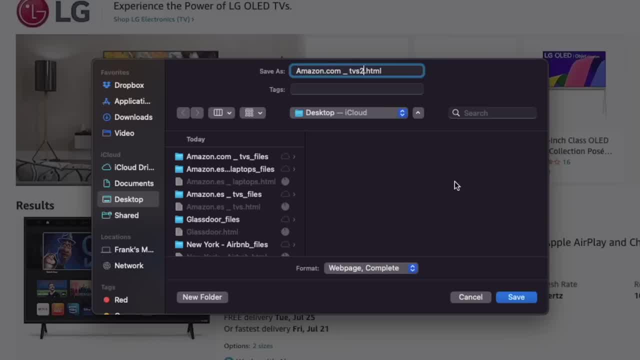 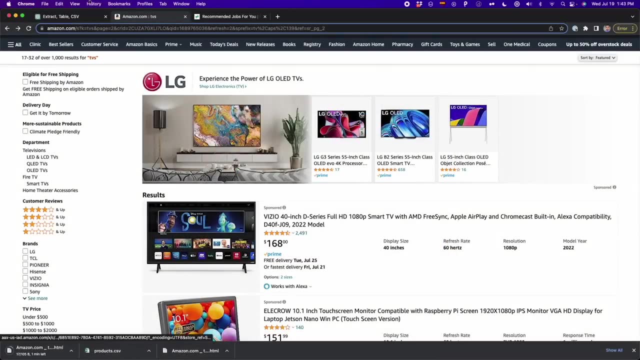 so here i press ctrl s to save this, sorry. so here now i press ctrl s. this is the second page, and now i'm going to write: amazoncom, underscore tvs 2.. so here i download this, and now it's done. so i have this file. then i go to chat gpt and 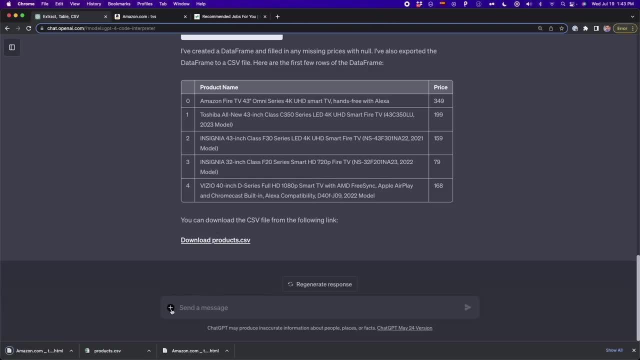 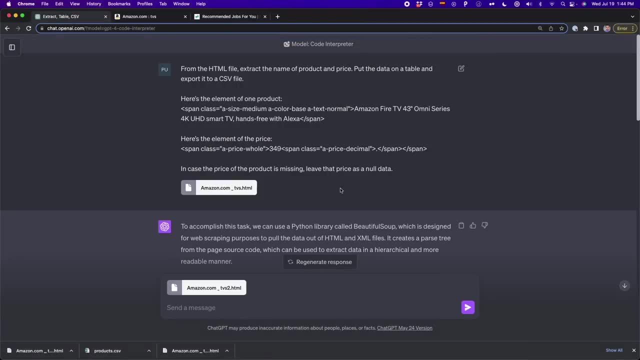 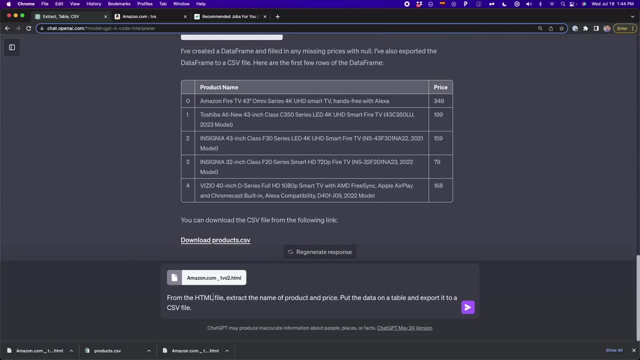 i'm going to upload this second page to extract all this data. so here i press on upload, then i upload this second page and now i'm going to the first prompt that i typed and here i'm going to copy this and i'm going to paste it. so i'm going to tell chat gpt that this is the second part of 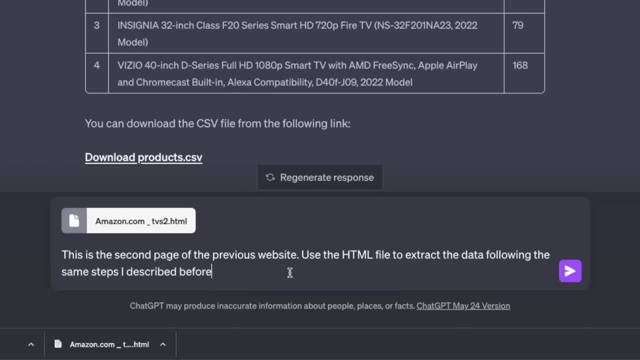 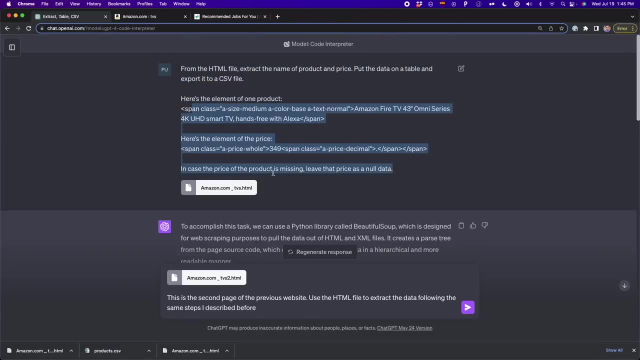 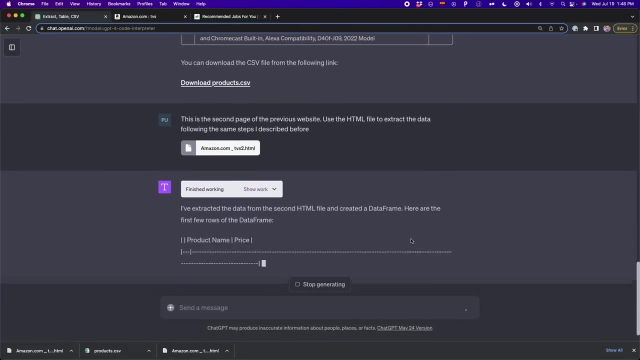 the website. so i type: this is the second page of the previous website. use the html file to extract the data, following the same steps i described before. so these are going to be the two different pages. so i'm going to press here and we're going to extract the data from this second. 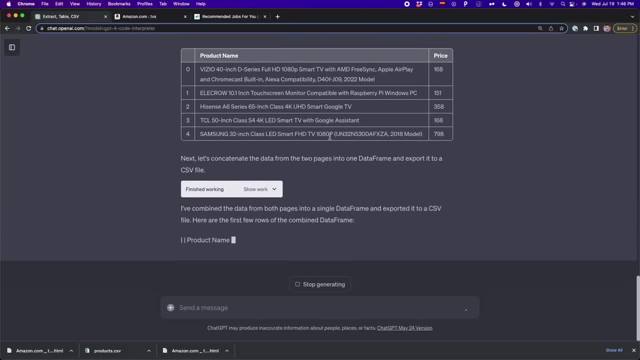 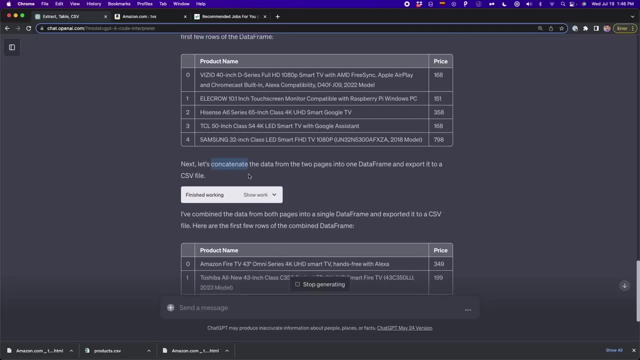 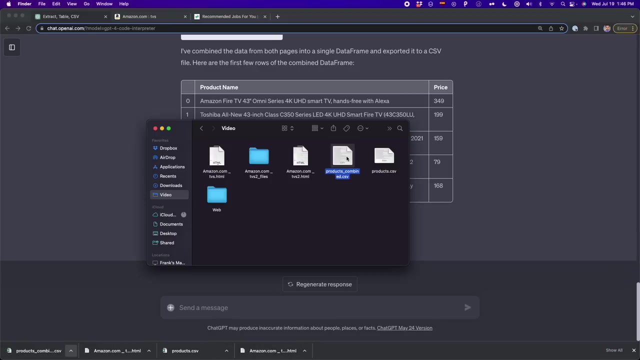 page. now, as you can see, it successfully extracted the name of the products in the price from the second page, and now it's concatenating the two pages into one data frame to export it into a single csv file. so now i want to click on download products combined. and now we're going. 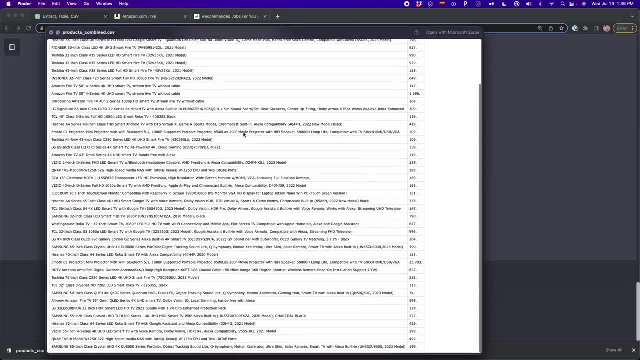 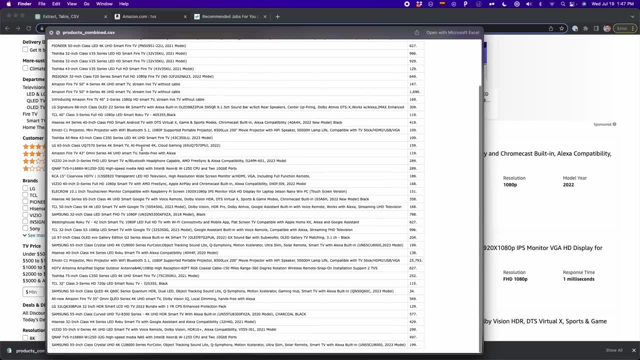 to have this file. now i'm going to open this file and we're going to see the preview and, as you can see, we have more rows. let's see here. the second page starts with vco for the inch, and if we can see here, we should. 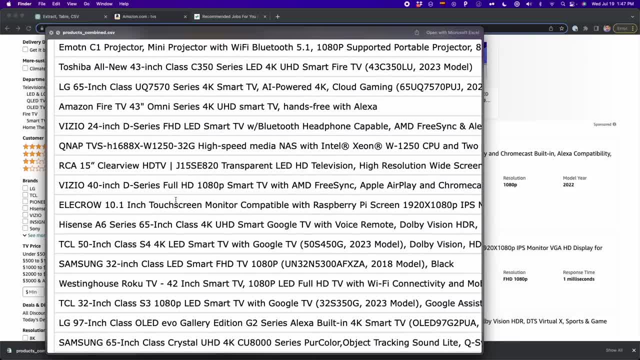 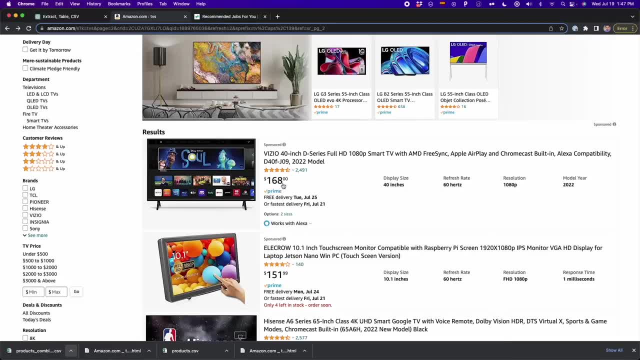 be able to find this product. so it's here: vco for the inch d series full hd, and the price is 168 if i'm not wrong, and here we can see the same name of the product and the same price. so we successfully scraped not only the first page but also the second page, and you can continue with this. 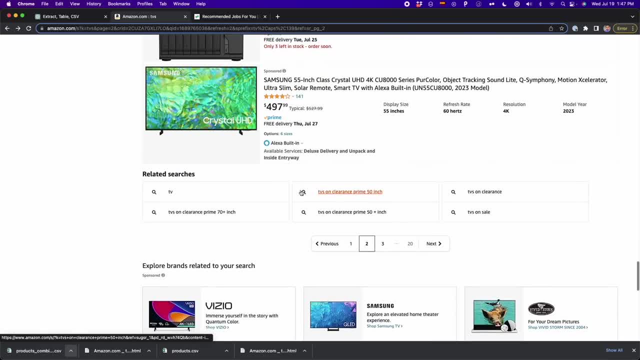 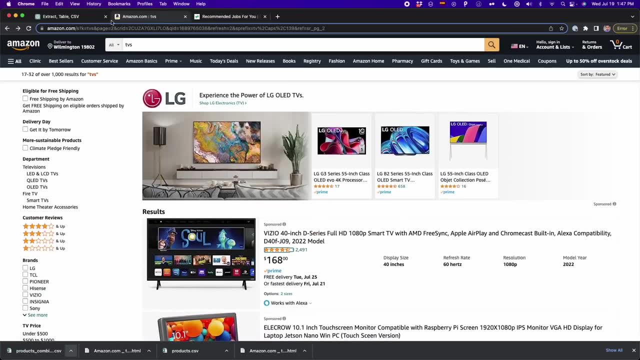 uh, with this process, with the third, the fourth and the fifth page, and as many pages as you want, and this is how you scrape data from amazon: using this approach with a code interpreter. now i'm going to show you another example, and in the second example i'm going to show you a slightly different approach to do web scraping. all right now. 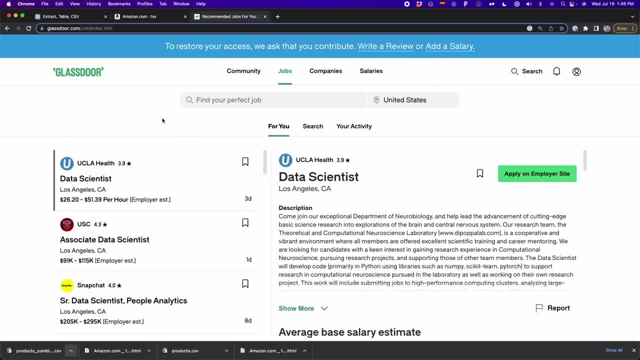 we're on the glassdoor website and here we're gonna extract the data that you see on the left. so here i typed data scientists to find jobs for that scientist, and what we're gonna do is something similar, but we're gonna do- uh, we're gonna use a different. 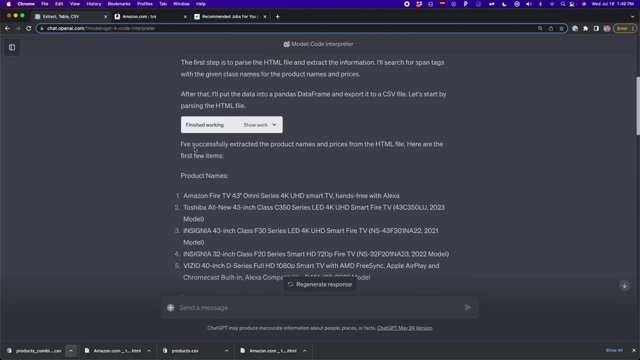 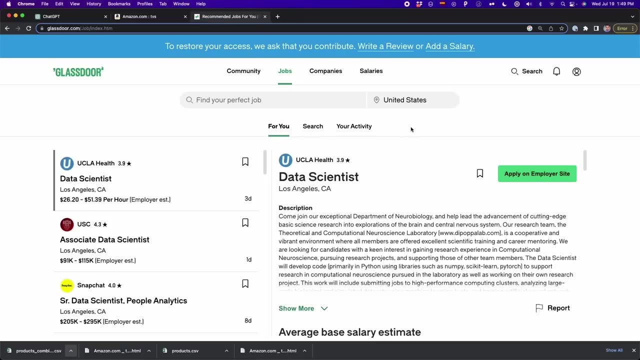 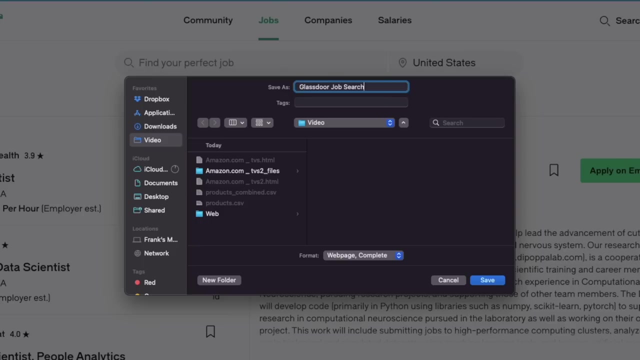 approach. so here i'm going to chat gpt again and i'm going to open a new chat and again i'm going here to glassdoor and i'm going to save this as html. so i press ctrl s, then i have this glassdoor job search and i'm going to type that html. so here, underscore ds for the designs, and then 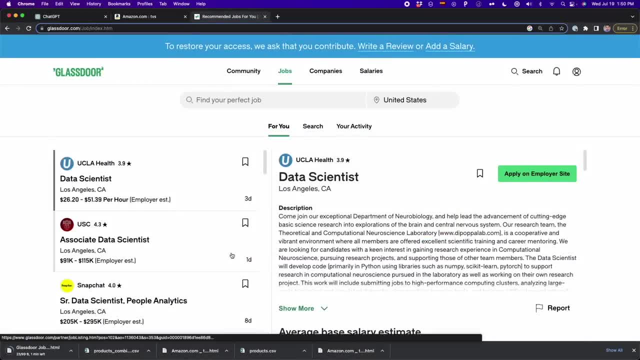 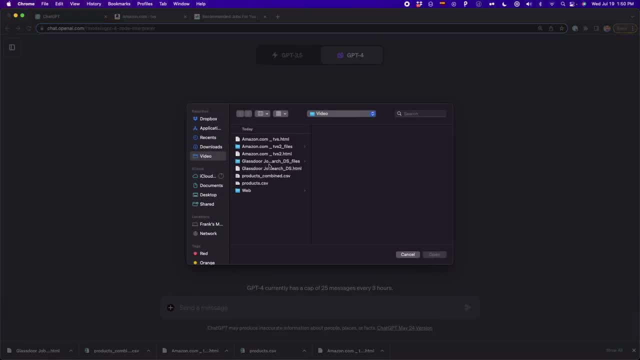 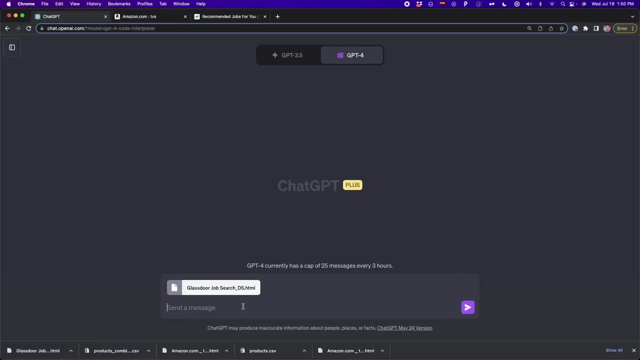 i'm going to save this and now we have this file. so once we have this file again, we go to gbt4 code interpreter and we upload this file. so, glassdoor job search dot html. i open this and we're going to use that following prompt, which is very similar to the previous one, but we have some. 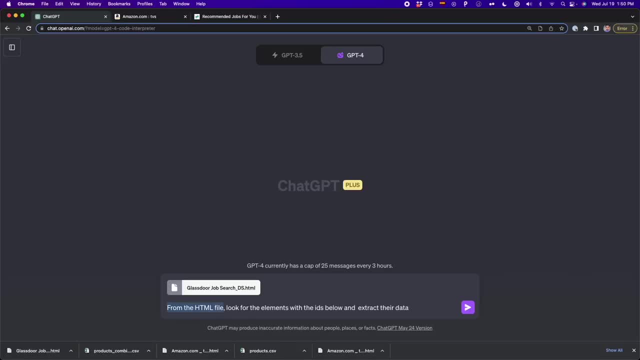 some other things that i'm going to add it. so, here, from the html file, look for the elements with the id below and extract their data. so i'm going to use the id as the identifiers for this. the elements that i want to extract and the elements: 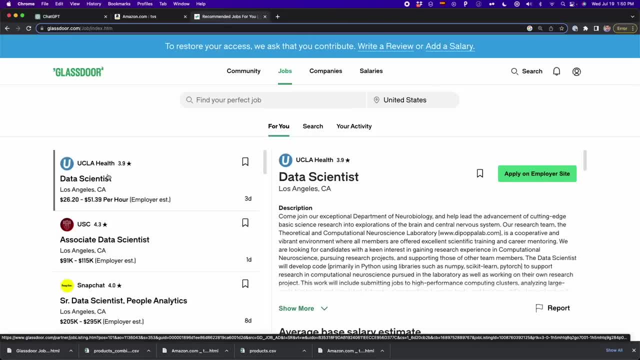 that i want to extract is the name of the of the company, then i also want to extract the job title- in this case data scientist- then the location and finally the job salary. and i can use the same approach i used before, which is right click, inspect and copy the element i want to extract. 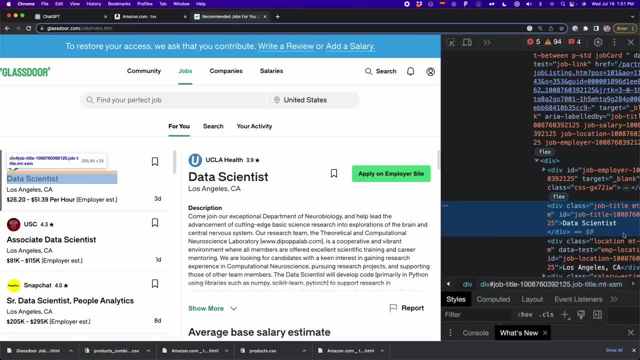 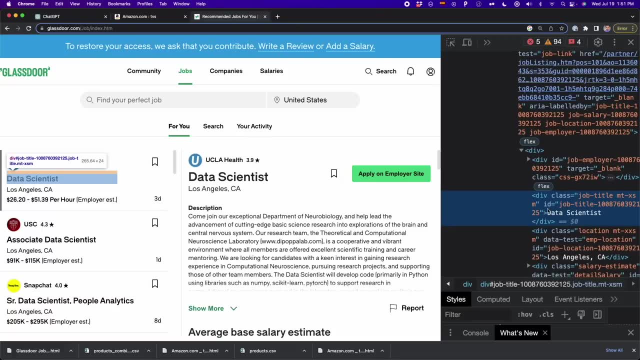 but sometimes it might not work. and in case it doesn't work, you can use a different approach, analyzing just the element that you're using. in this case, i have this element and here, as you can see, there is an id, and this id has a very clear name: job. 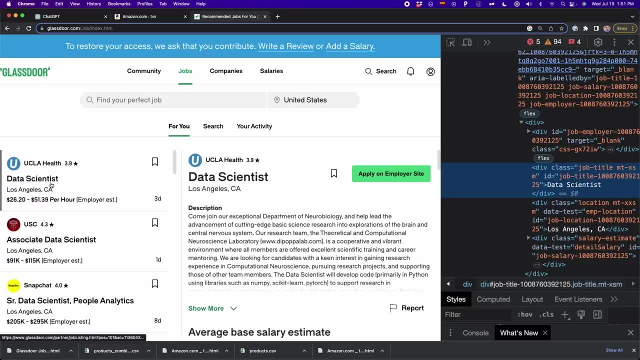 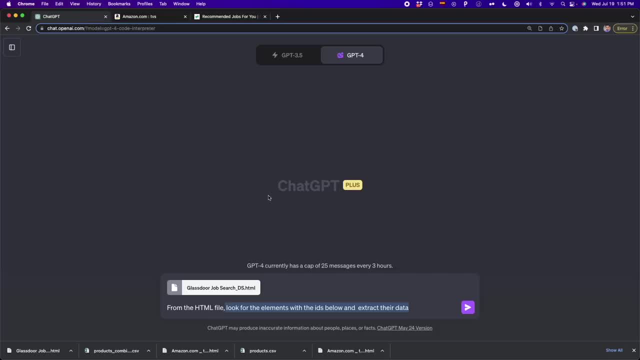 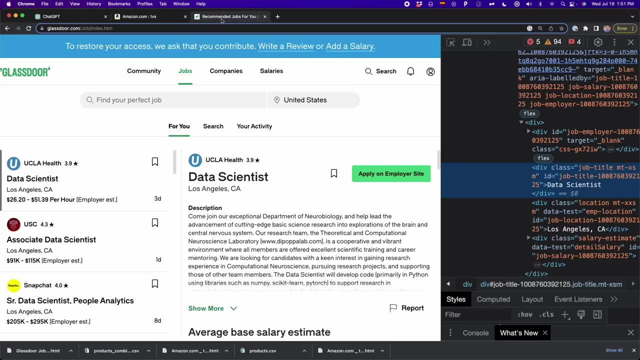 title and this job title represents the name of this job, which is data scientist. so here, if i copy all this, the name of the id, i can just list all the ids i want to extract. so i started with the job title, then i can continue with the company, the name of the company. so here i can go to job employer. 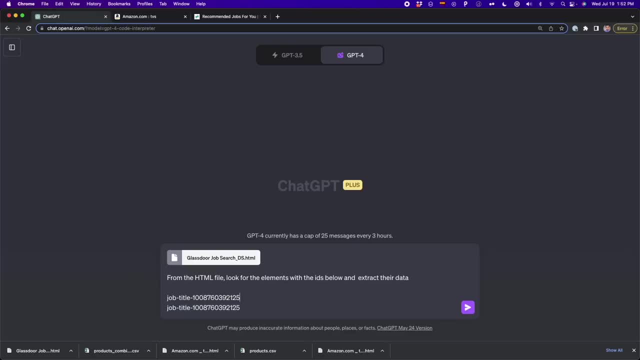 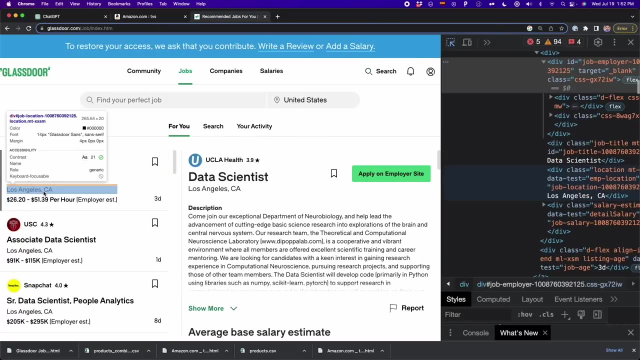 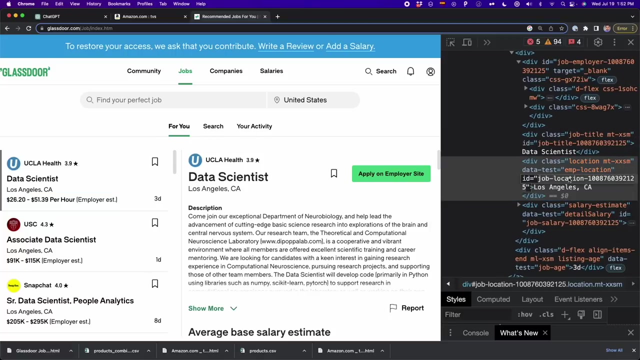 and paste it again. so here, instead of job title, job employer, and then i want to continue with the location and the salary. so here: select again the location, then i'm going to use the id which should be here. so id, job location, just copy and paste it. we have one more, which is the salary. 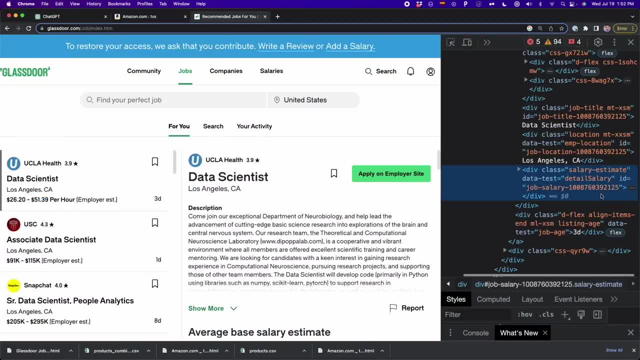 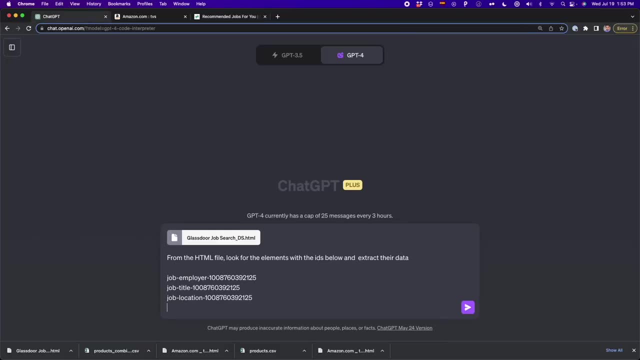 and again just select the salary and then the id. actually you can use another element, not necessarily id. i'm just using the id because it's unique, but you can use the data test attribute or the class. it might work. it might also not work, but it depends on the website that you're. 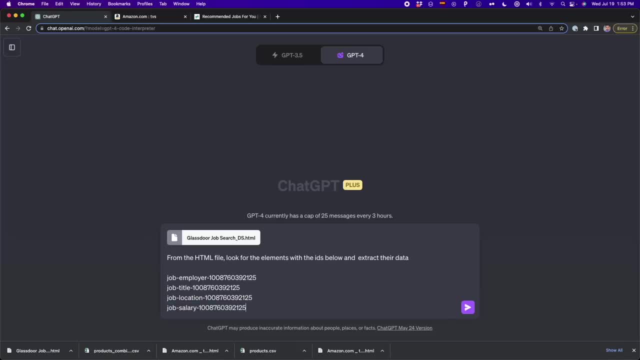 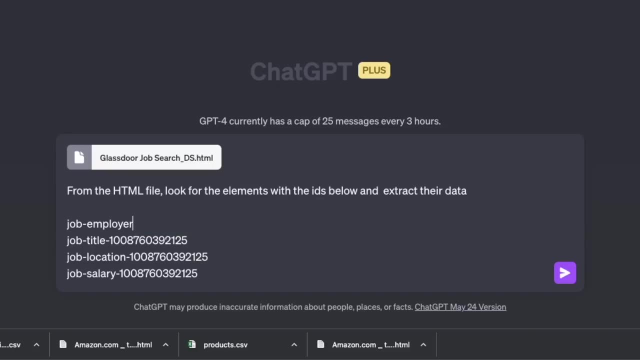 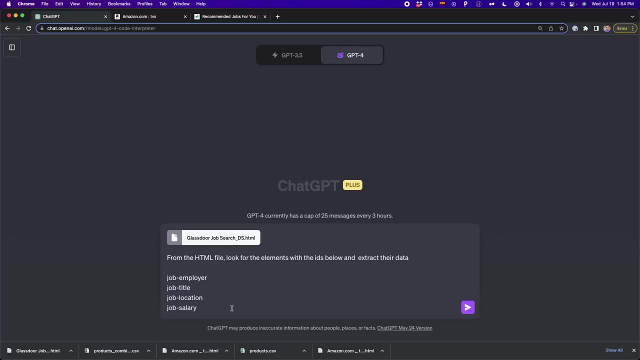 scraping. so here, finally, i have job, salary and, as you can see, these ids have these numbers which are not necessary, so i can delete these numbers again. you can simply copy the whole element and paste it, as we did before, but in this case we're only using these words. 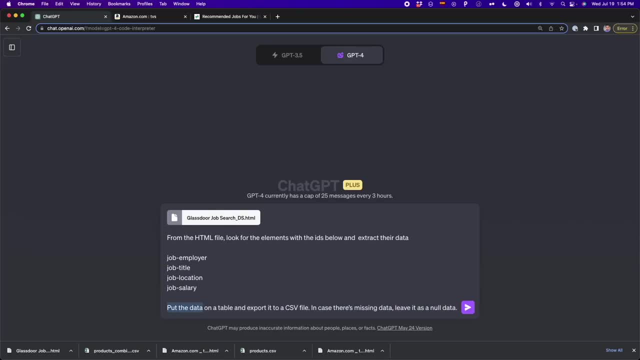 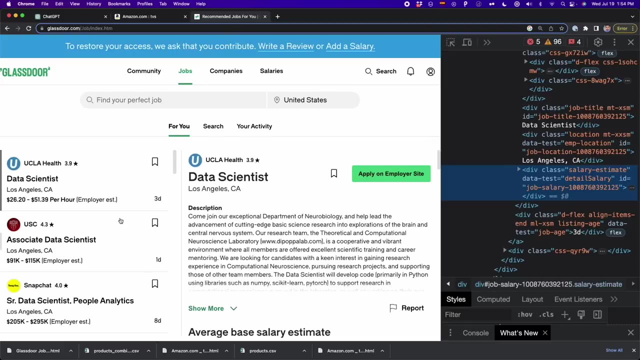 and now i'm going to tell chatgbt that- to put the data on a table and export it into a csv file and in case there is missing data- because there are some companies that don't have the salary here, that, for example, this one doesn't have the salary- 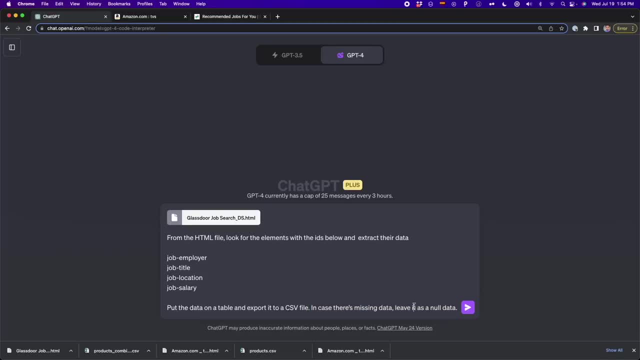 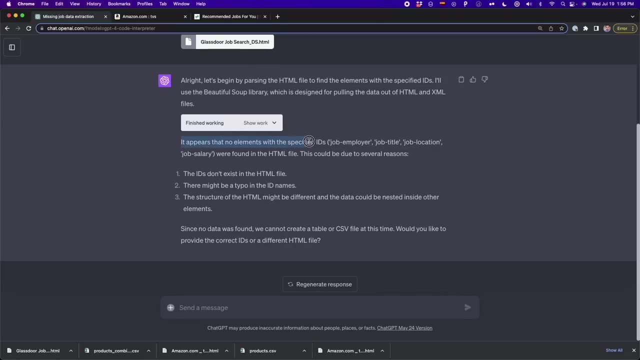 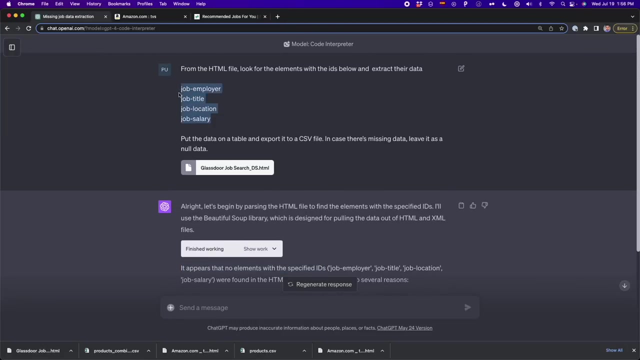 so, in case there is missing data, just leave it as null data. so now i press enter. now chatgbt says that there's no element with the specified ids, and that's true, because i deleted the rest of the id and i only left these words, and what i can tell chatgbt is to use regs to match. 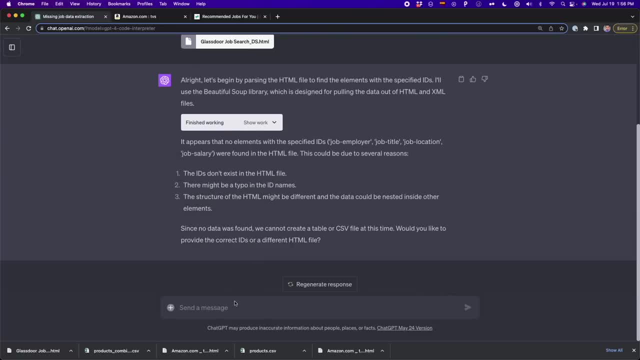 that part of the id. so i'm going to type the following: so those are parts of the id. use regs to match that part of the name of the id and with this chatgbt it's not going to match exactly the whole name of the id. that is going to verify that if the id contains. 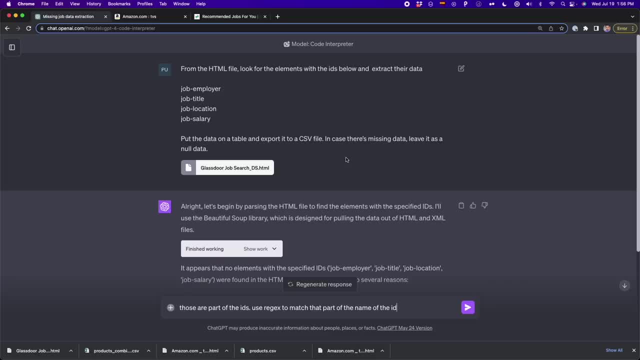 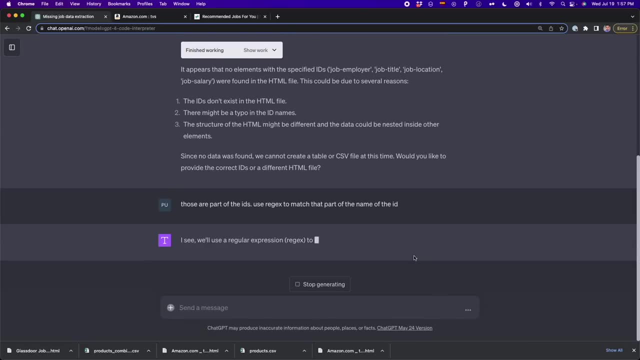 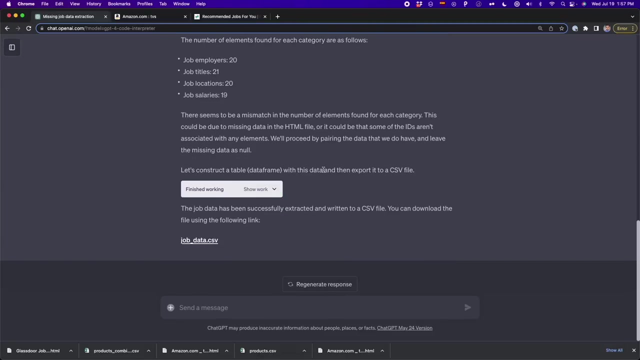 these words- job, employer, job title, location and salary- is going to be enough to match to extract this data. So here I'm gonna tell this and hopefully we're gonna be able to extract the data that we wanted. So, as you can see, ChatGP destroyed all the data. 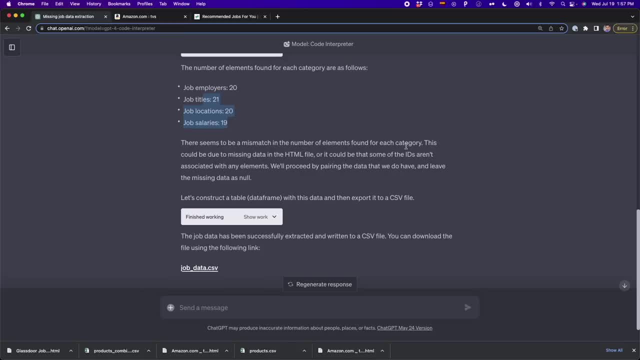 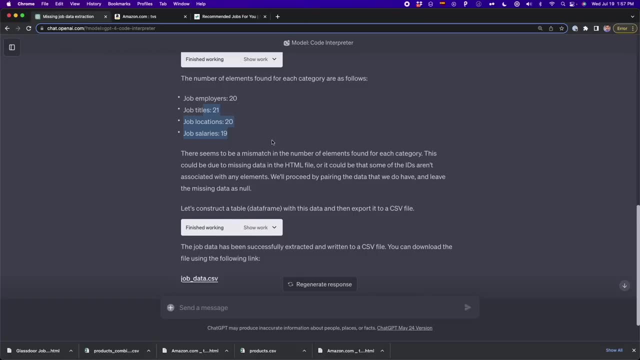 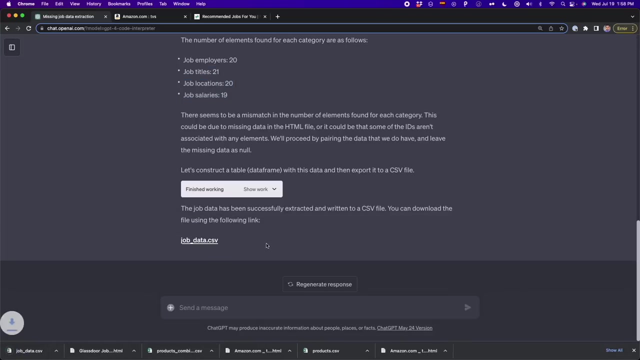 and even told me that there is some mismatch in the number of elements found for each category. So hopefully it left the data point as null and it didn't duplicate any job title or location or salary. So we're gonna verify this. I'm gonna download the CSV file.